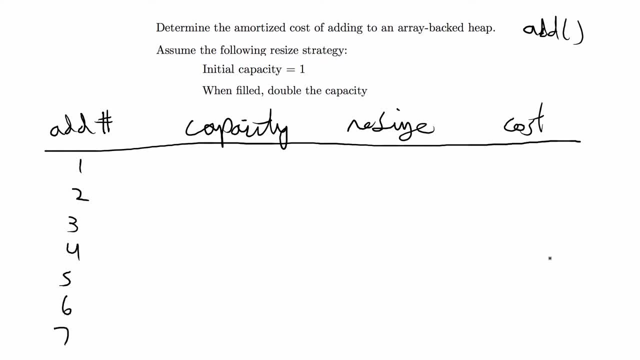 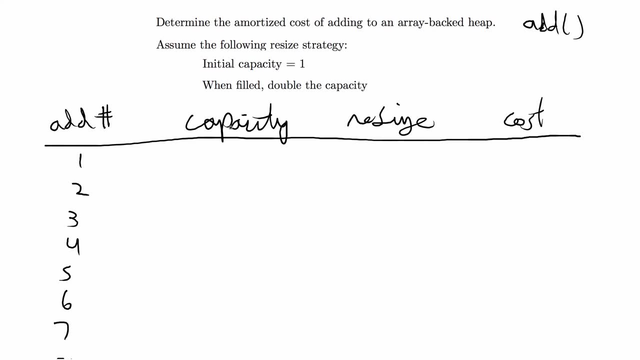 enough times until we can find a pattern. So I'm going to go up to nine and we are given enough information to know what to do with the capacity, the resize and the cost. So the first time you're adding to the array, the array is empty and it has a capacity of one. You don't have to resize. 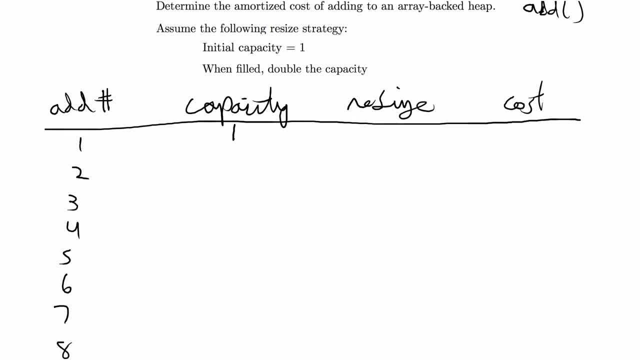 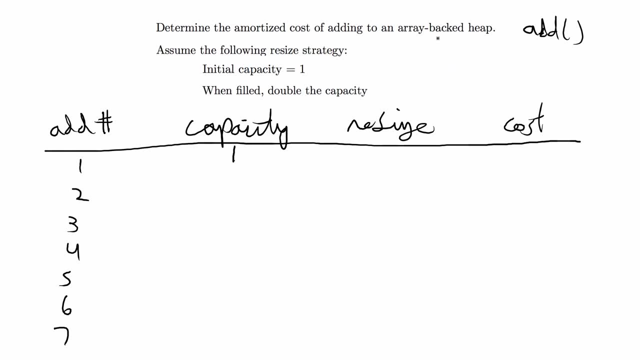 because all we're doing is adding for the first time and we're just going to say that we know, or you should know when you're doing this, what the cost of adding to an array heap is. So that's going to be, in general, it's o log of n. So when you're adding one, the cost is going to be log. 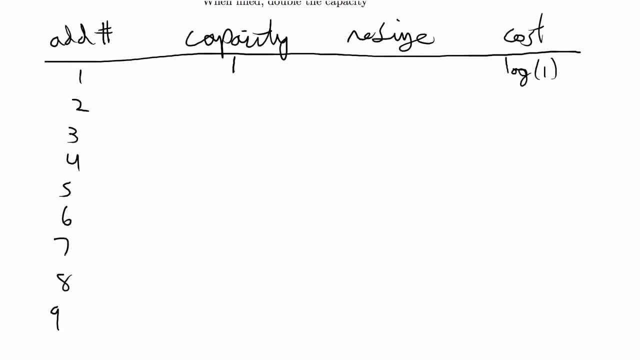 of one, and so we're done with the first one. Now to add a second to the array we have to resize. so we have to do our first resize. The capacity is now going to be 2, because we know from the strategies that we double the. 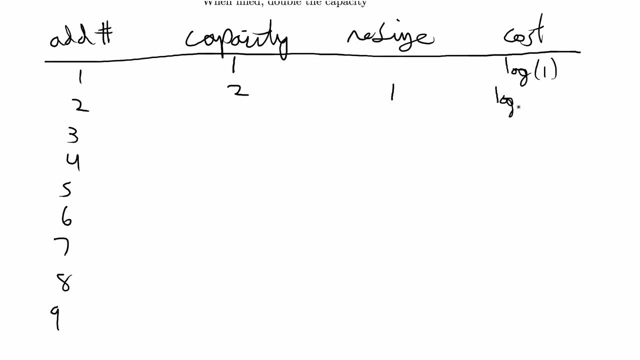 capacity when the array is full, and so the cost is going to be the cost of adding. our n is 2 here, so it's log of 2 plus the resize cost is 1.. We have log 2 plus 1 for adding a second item. Our capacity is 2.. To add a third item. 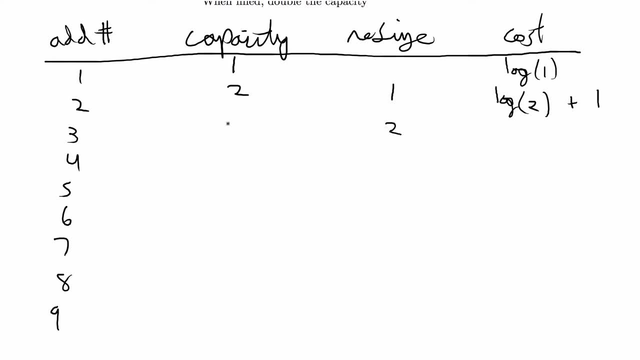 to the heap. we're going to have to resize again. so now our capacity is 4 and the cost is going to be log 3 plus the cost of adding 2.. We don't have to resize to add 4, so our capacity is still 4.. We leave this blank and it's going to. 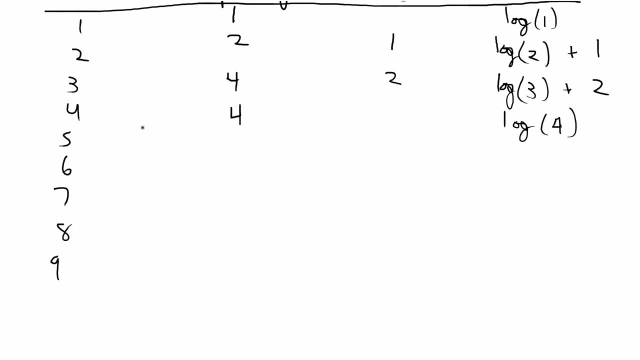 just be log 4 for the cost For 5. we're going to have to resize again because our capacity was 4. so we resize and add 4, so our capacity is now 8.. Now we have 3 extra items that I have to add for the heap. This is going to be: 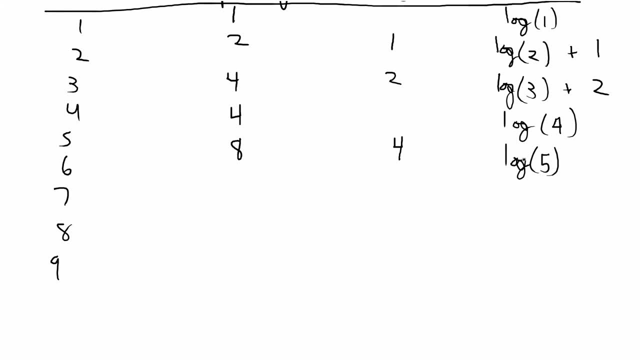 and the cost of adding five is going to be log five plus the resize cost, which is four, And so now we're going to be able to add up to eight without having to resize. So our capacity can stay at eight, We don't have to resize. 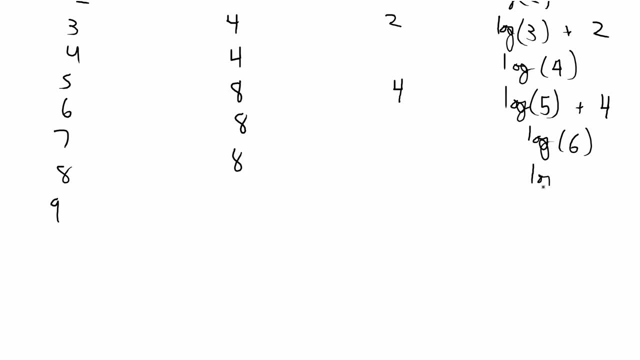 This is going to be log of six. This is going to be log of seven. Eight is still going to be just log of eight, And then we're going to do one more final resize. So to double, we're going to add eight.